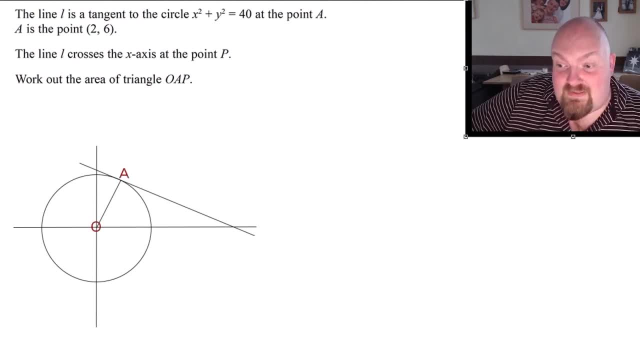 the origin. we have A, where the tangent meets the circle, and we have P, where the tangent line crosses the x-axis. Okay, Here we go, here we go, here we go. bear with me, right, okay. So, first thing I'm going to do with this question, I'm gonna just label a couple of other. 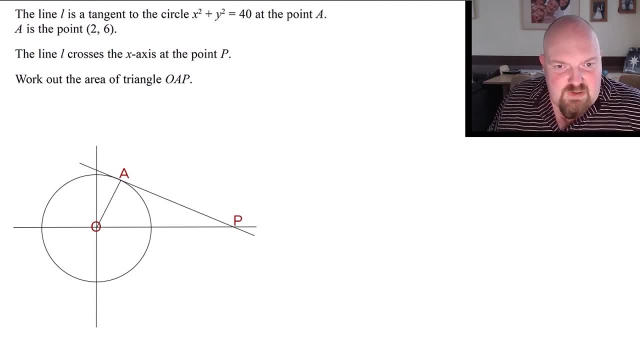 bits. okay, Like we said, we don't do F, they are Cuzou's. were going to need to um, we don't need to measure too much of it, but there are a couple of bits that would be really helpful to just label. so the first is that that there is six and that there is two, we know. 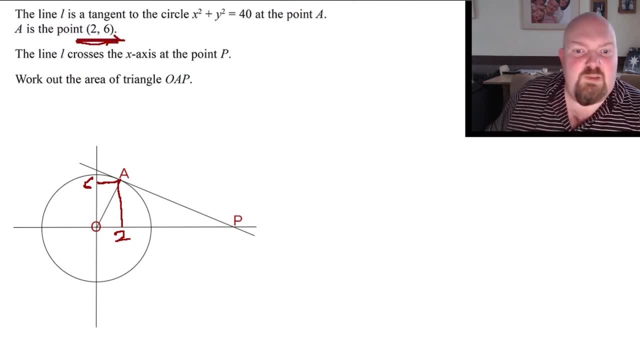 that, because the question includes this point. once i've got that, i can then work out the gradient of the point of the line o a, and the gradient of the line o a is six up for two across. six, divided by two equals three. we'll need that, because what we're then going to do is we're 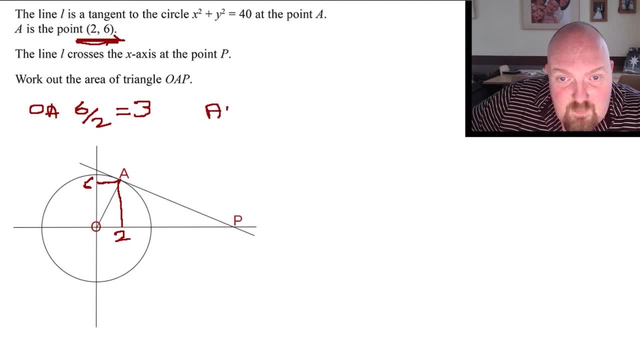 going to work out the gradient of the line a, p now. you'll remember from your lessons that, um, if two lines are perpendicular, then there's a special relationship with their gradients. so, um, the way we work out the gradient of a perpendicular line is that it is negative one. 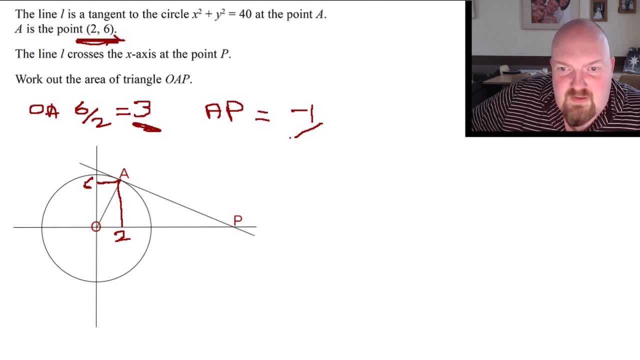 over the original gradient. so in this case it's going to be negative one over three. okay, um, so just to recap with that: if two lines are perpendicular, then the second line has a gradient that is negative, one over the first gradient, right? so we've got this. now we can then, because ap is a 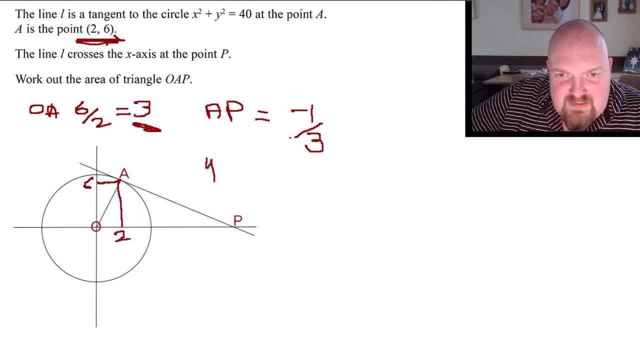 stretch line straight line. we can then start to plot it as y equals mx plus c. we can fill three of these things in. we know the gradient m is negative, one over three. we know that y, that one of the points, this point here, uh, what that? at that point we have y equals six and x equals two. so i know that six. 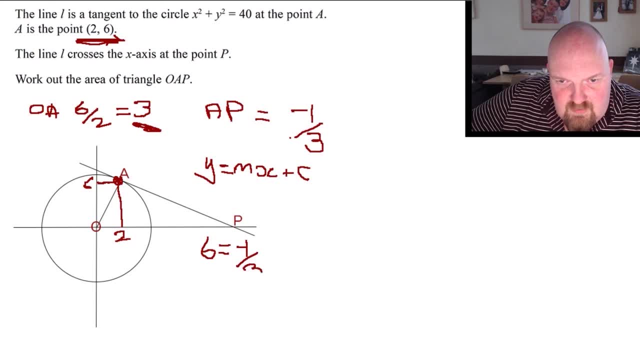 equals negative one over three times two plus c. okay, a little bit of simplifying. we get six equals negative two over three plus c. and then by simplifying further- so we uh, cancel this down, so we bring this across- we get that six and two thirds equals c. okay, 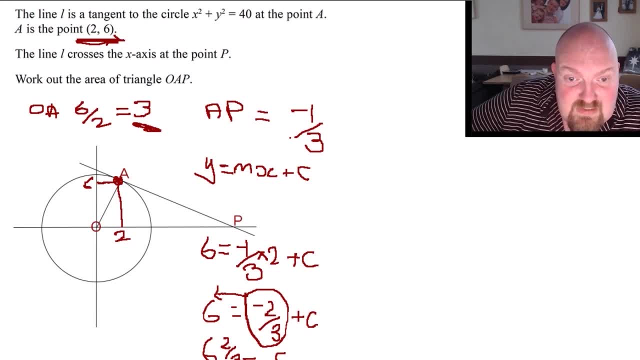 i can now take that and i can then put that back in to get the the proper equation of this line. so this line is: y equals negative, one over three, x plus six and two thirds. okay, i've now got that point. so we're now heading really close to being able to solve this, okay. 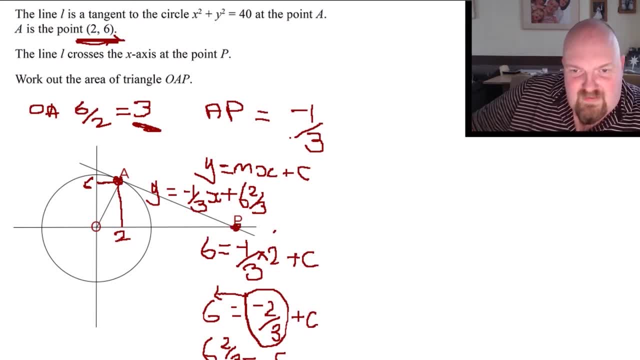 because of that i can work out this value here. and this value here is where um, where the um, where the line crosses the x-axis. so if the where the line crosses x-axis, the y value is zero. so i can rewrite that again now and i'm going to say that zero equals and negative one over three. 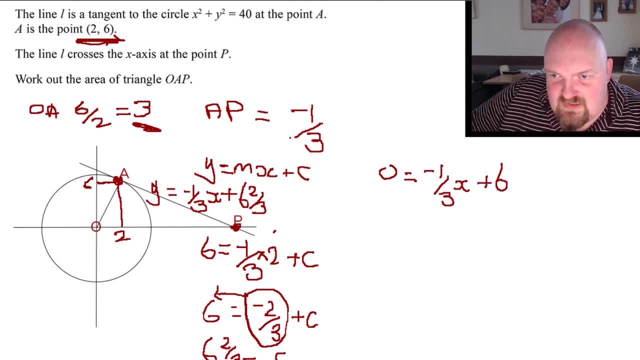 x plus six and two thirds. with a little bit of um rearranging i can take this across to the side so i can get change the side to 90 and i can say: here's my x and the negative two form up so i can get x over three plus n and i can put this back in to get the negative one over three, x plus six and two thirds. 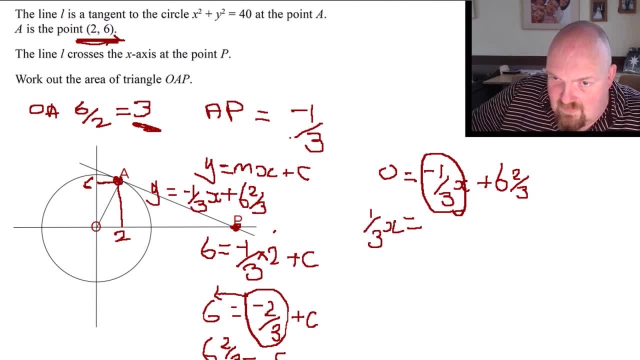 range. and if i could retained this- and now we're going to sort this across to the one side so i can get change the sign- so a third of x equals six and two thirds. if I then multiply both of those sides by three, I get that x equals 20, okay, so now that I've got this value, I now know that the coordinates. 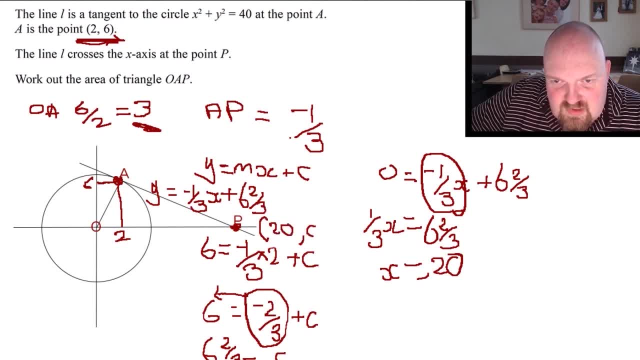 of this point are 20: 0. okay, so we've got a lot of what we need there. okay, I know that let me just draw this out again which we're going to go really badly and you'll then see why I am. why I needed to definitely use the um, the computer, to draw the main. 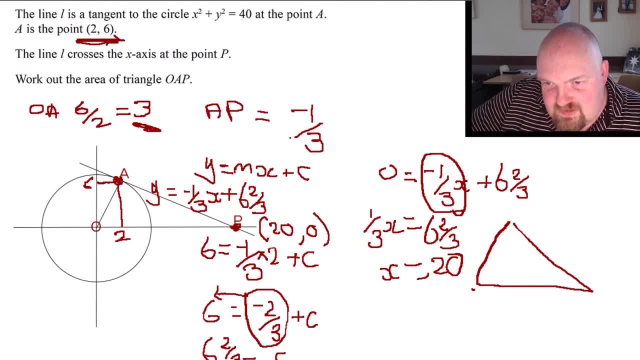 diet of the main sketch. so I know that this point is zero, this point is 20, so that length there is 20. I know that this that the vertical height is six. so because the vertical height is six, then all I need to do to work out the area, of course, is I use the, the formula base times height. 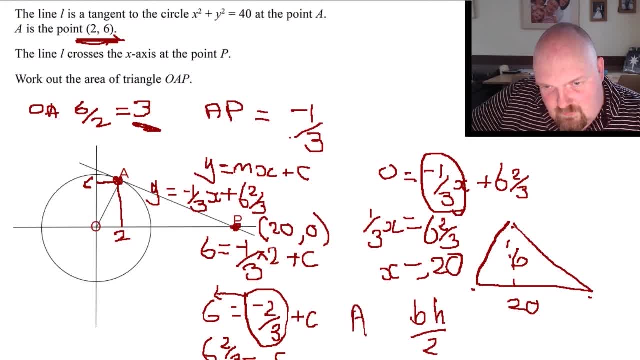 x, x, x, a divided by two, so that's the area, equals. so base is 20 times six divided by two, and that's my area. 20 times six is 120. 120 divided by two is 60, so the area, so the area of oap, is 60. 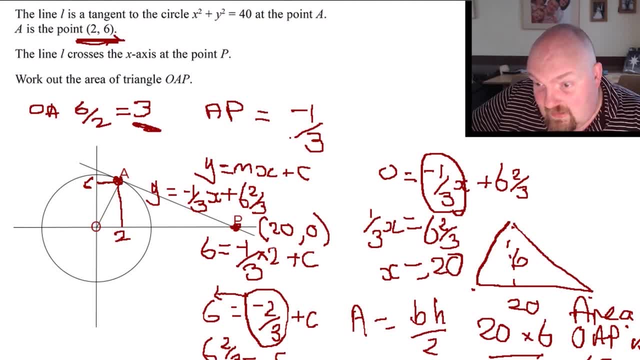 units squared. okay, and there is your answer. okay, now lots and lots steps. I appreciate that I've gone through that quite smoothly, but, um, there are lots of steps and there are lots of things that you could do. that will get you confused, that will get you mixed up. the good news is, with this one. 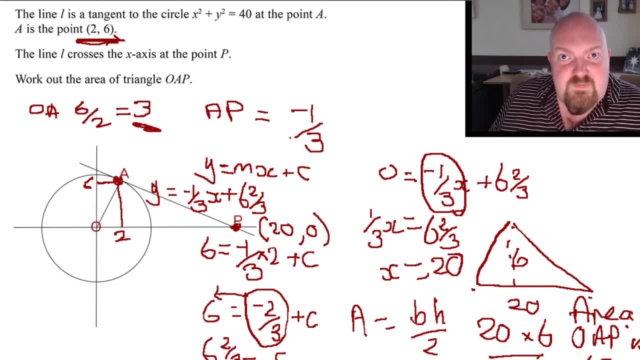 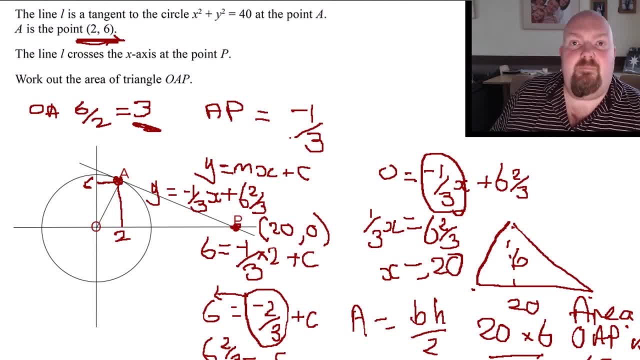 even if all you can do is put the sketch in, depending on the exact nature of the question, that might go some way to getting you a mark. the worst thing you can do with any exam question is to run away from it and hide. okay, because that's definitely not going to get you marks. 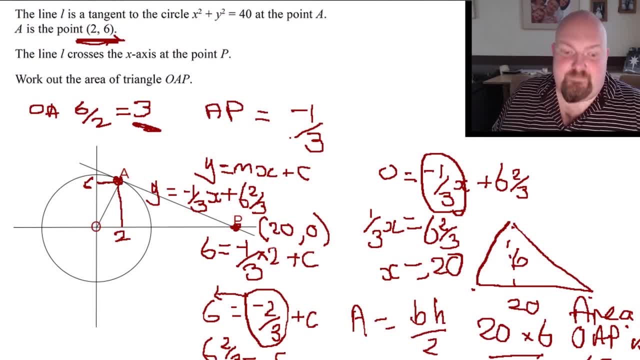 you put anything down, there's always a chance, okay. so so there we go. so that's that question. I hope that all made sense. hopefully, as you follow it through, you'll see where my little scribbles appeared and will be alright, and but yeah, so, like I say, taking it to to the extreme now that's one of the the harder. 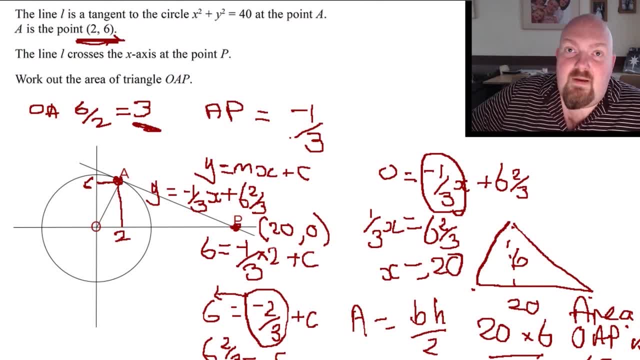 questions that you're likely to find in your GCSEs. okay, guys, thank you so much. I'd love to hear some, some requests. I'd love you guys to send in some problems that you've got. please do so and we'll see if we can work on them, okay.